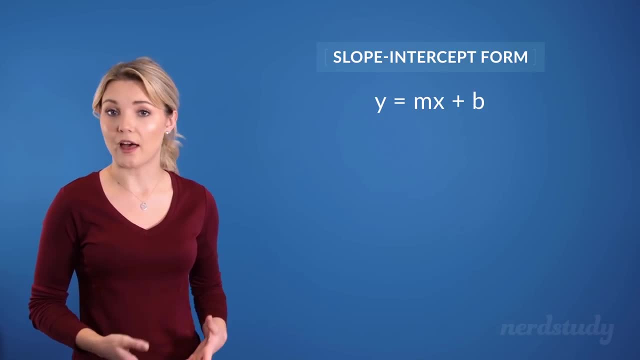 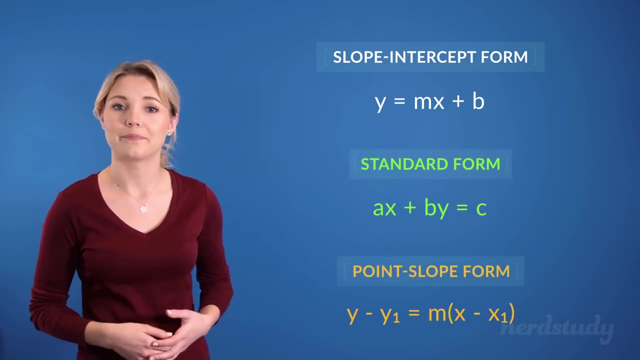 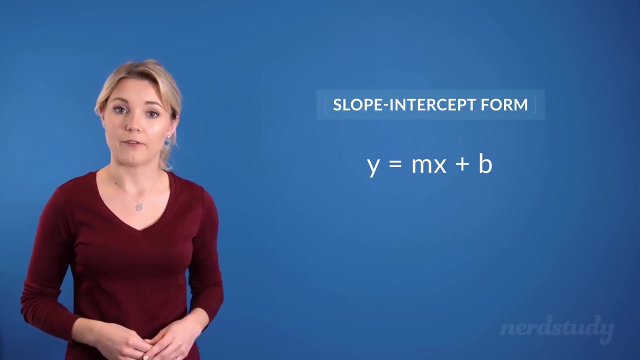 Well, there certainly are other forms of linear equations that express the same line, only that they express them in different ways, such as the standard form and the point-slope form, But we'll explore those forms in another lesson. Just remember that the slope-intercept form follows this format, where we have our y isolated. 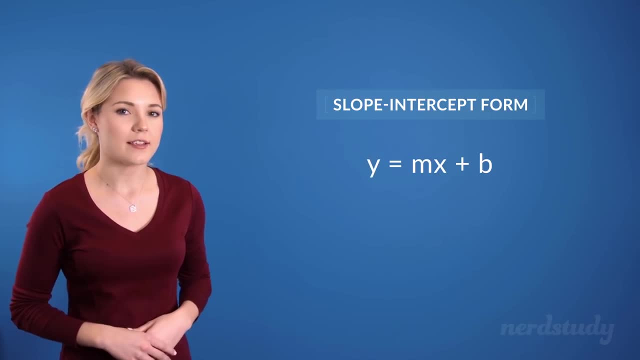 onto the left side. Now, what's interesting about the slope-intercept form is that when the equation is simplified down to this, the y is isolated onto the left side. So the slope-intercept form has the y on the left side. Now what's interesting about the slope-intercept? 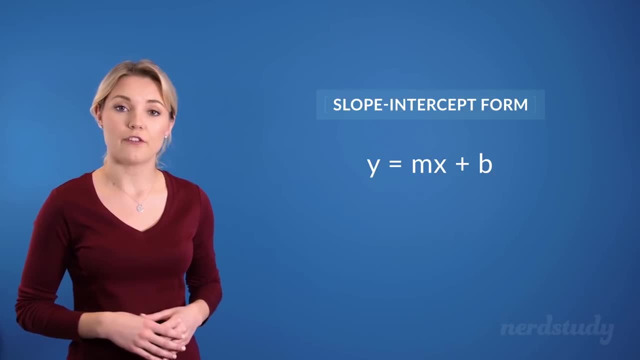 form is that when the equation is simplified down to this state, it makes it easy for us to identify the slope of the equation and the y-intercept. In this form, the slope is always equal to this m, right over here, and the y-intercept is equal to b, hence why we 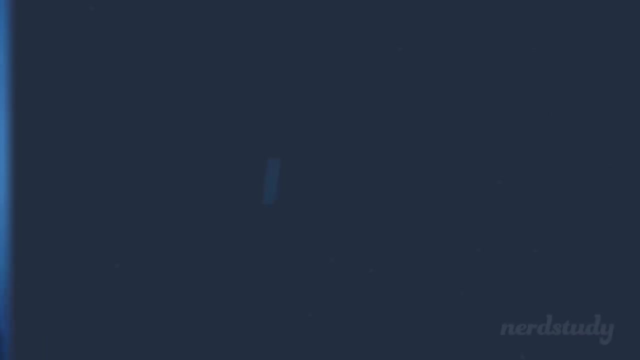 call this form the slope-intercept form. So what do we mean by y-intercept? Well, the y-intercept is the place in which the line will intersect the line. So the y-intercept is the place in which the line will intersect. 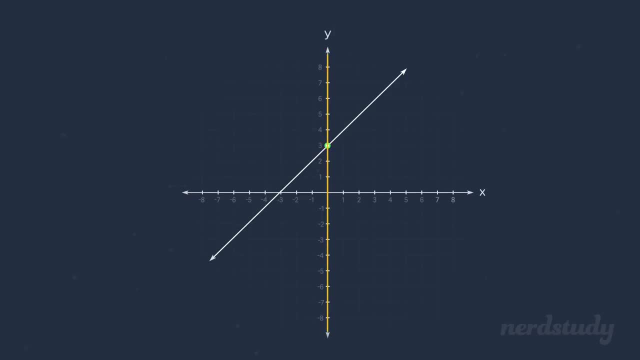 the y-axis. Remember the y-axis is at a place where x equals 0.. So in a graph like this one, when x equals 0, y equals 3, making our y-intercept equal to 3.. And in this graph, 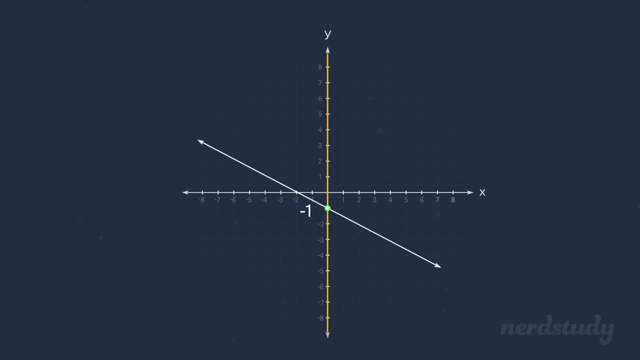 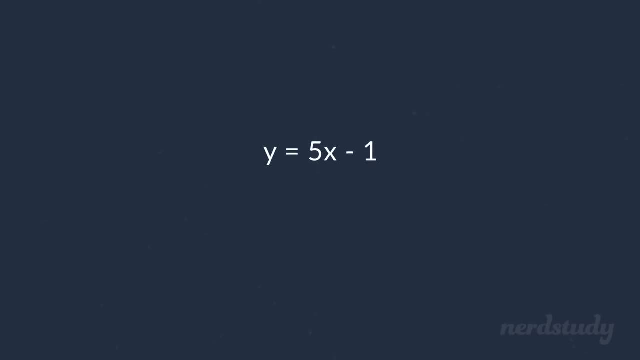 So the y-intercept is the y-intercept, So the y-intercept is the y-intercept. so, for this equation, what would be the value of the slope and the value of the y-intercept? well, remember, the slope is the value in front of the x when y is isolated. so that would be 5. 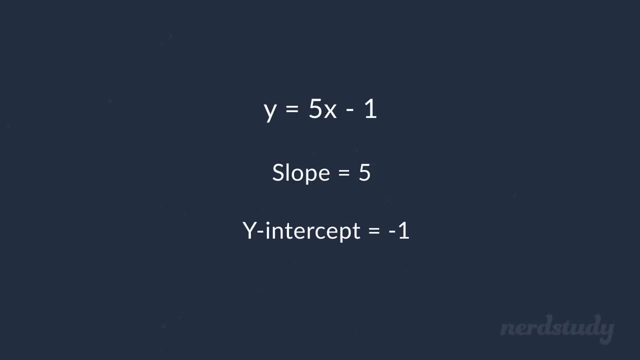 and the y-intercept would be negative: 1. good, now, that was pretty easy, right? well then, let's imagine that we've got a linear equation like this one: two different students give their answers to what they think the slope and y-intercept for this equation would be. it's now your turn to determine who has the right answer and who has. 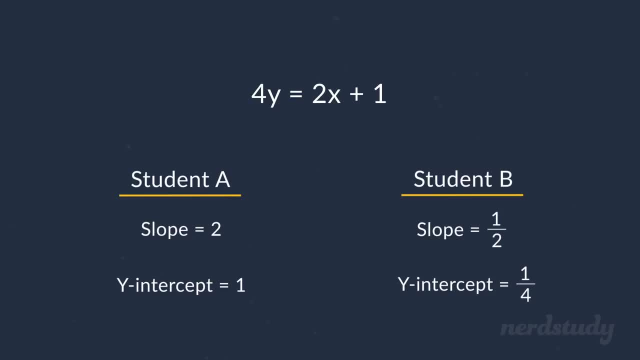 the wrong answer. well, in this case, student b has the right answer. now it's important to be careful here. some people might assume that the slope and y-intercept would be negative 1 and the y-intercept would be negative 1 and the y-intercept would be negative 2. so we assume right away that the 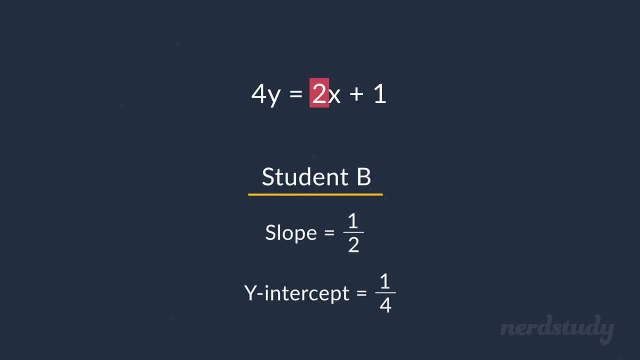 coefficient number right in front of the x variable is automatically the slope. but this is only the case when we've already isolated the equation to have the y variable alone on the left side. in this situation we've got to first divide both sides by 4 to isolate for y to get the 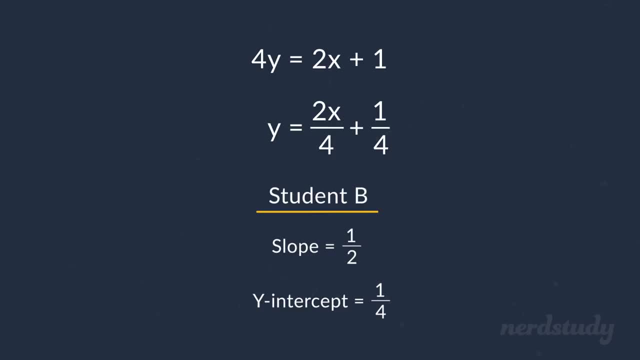 following, of course. now our slope would simplify down to just 1 over 2 and our y-intercept would be 1 over 2 and the slope would be negative 1 and the y-intercept would be negative 1 and the slope would be negative 1 and the y-intercept would be negative 2 and the slope would be negative 1 and the 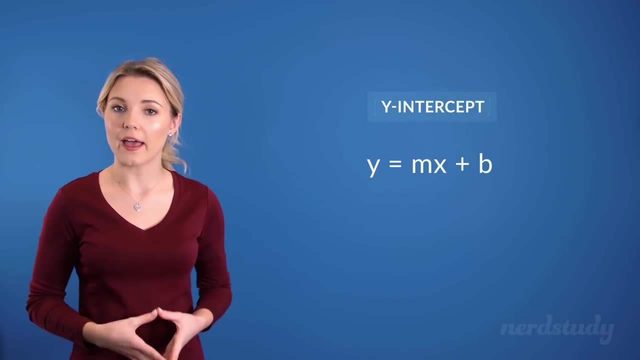 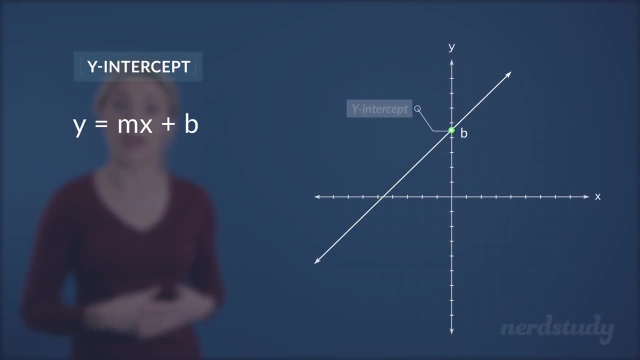 slope would be negative 2 and the slope would be negative 3 and minus 2. write over 4. now we know that the y-intercept can be identified by the b variable here and that this is the point where the line intersects the y-axis when x is equal to. 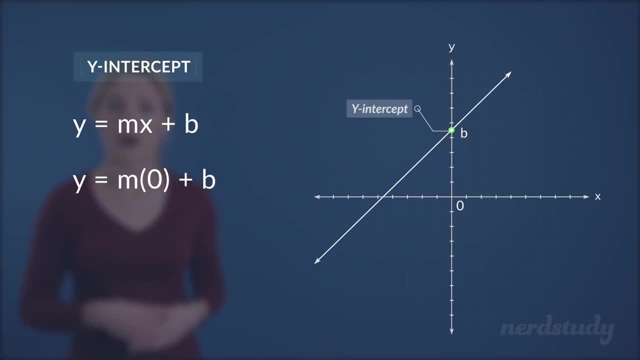 0. if we wanted to actually test this out, we would substitute 0 for x and notice how, regardless of what the slope would be, we would get. What this means is that if we were given a table of coordinate values and one of the points have an x value of 0, then we can expect that the y value to automatically be the y.